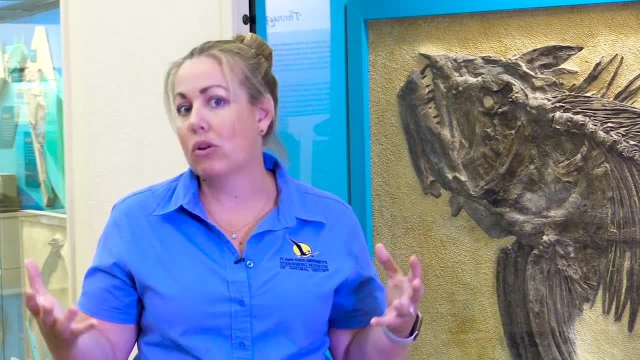 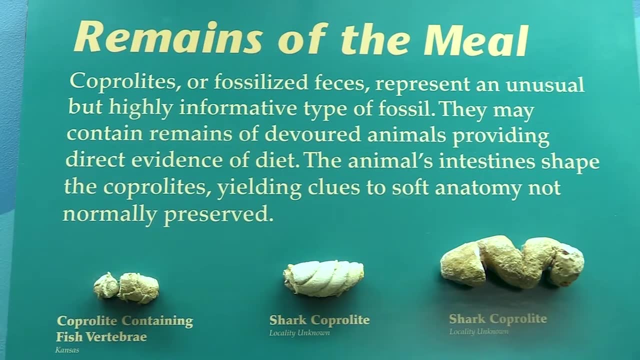 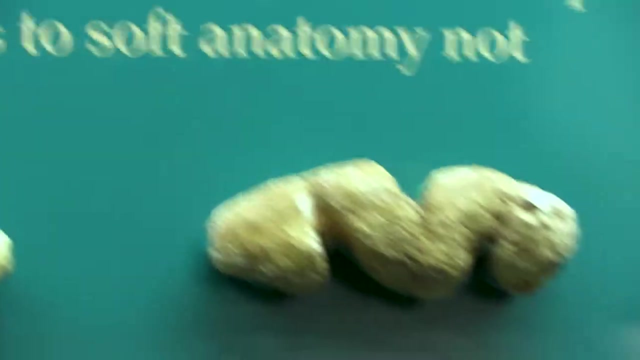 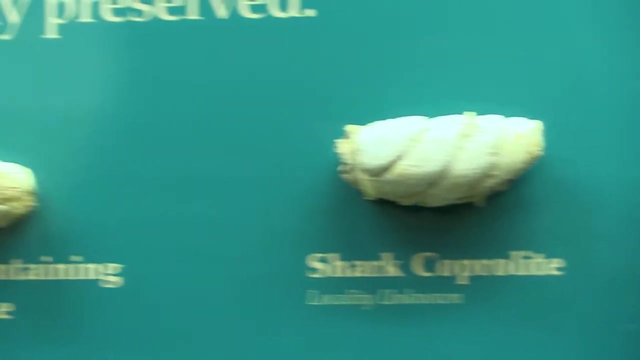 There are other pieces of evidence that we can use to help elucidate or clear up some of these ecological relationships, And one of those is using coprolites, or coprolites, And these are fossil feces, so actual fossilized poop from different animals. And we can go and look at those fossilized poop- they don't smell, they're rocks now- and actually look for pieces of possible food items in there. So whether it's fish bones, whether it's pieces of crab or lobster, whether it's 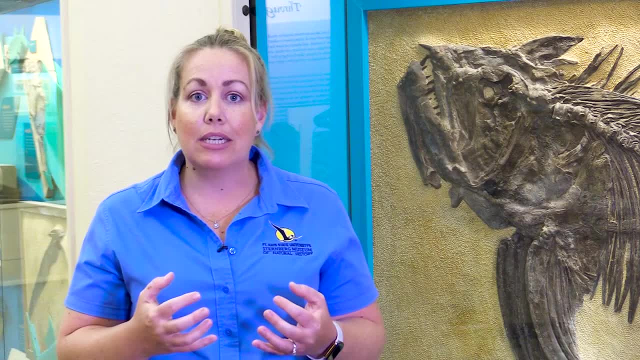 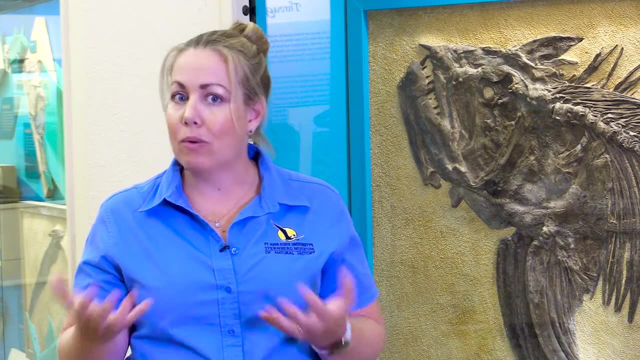 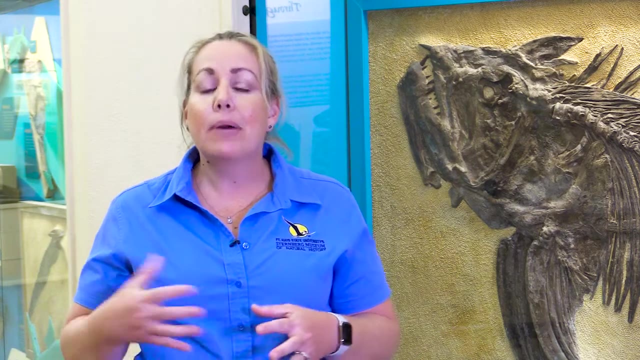 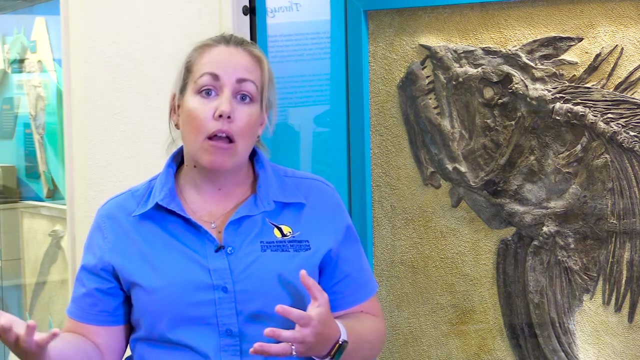 pieces of clam shells. So we can actually see what was being eaten And if we're really lucky we might even know who was eating it. So one of the hardest things for figuring out with coprolites is who actually pooped that poop. That's something that's a little bit harder to figure out, But again it's evidence of the different size of organisms and the different types of organisms that were maybe eating other things within the ecosystem. Sometimes the fossil record will make it a little bit hard to 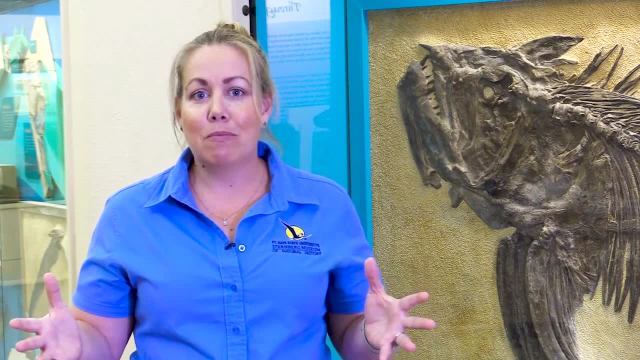 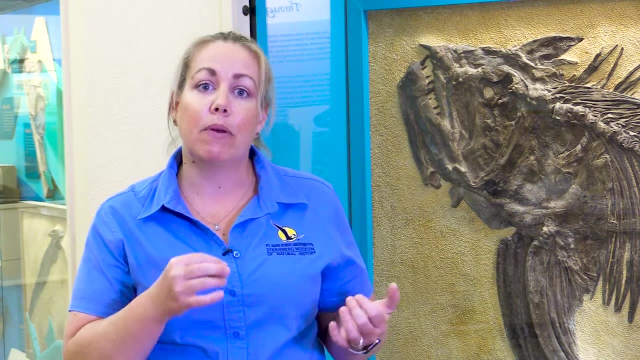 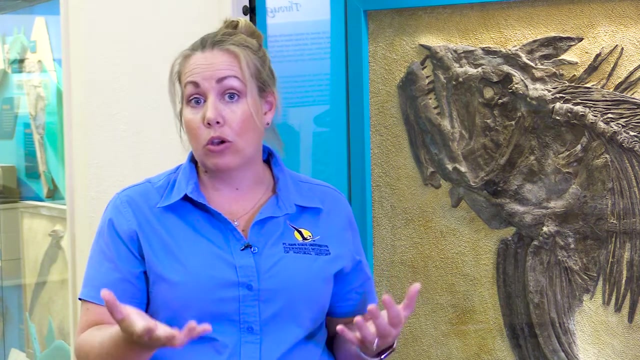 harder on us and we have to go back to just using old fashioned anatomy, So looking at how an animal is put together, so how the size and the shape of the bones would have fit together, So what that animal would have looked like, and then how or what it could have eaten, So we can go back to our 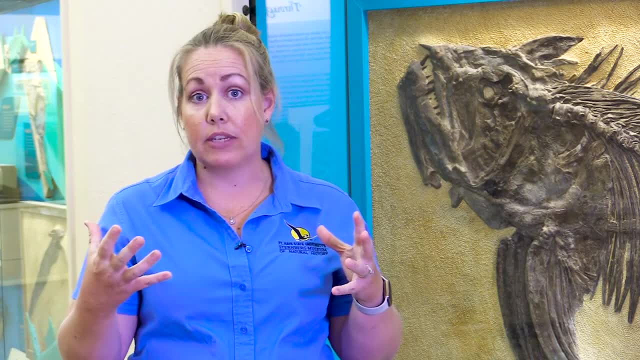 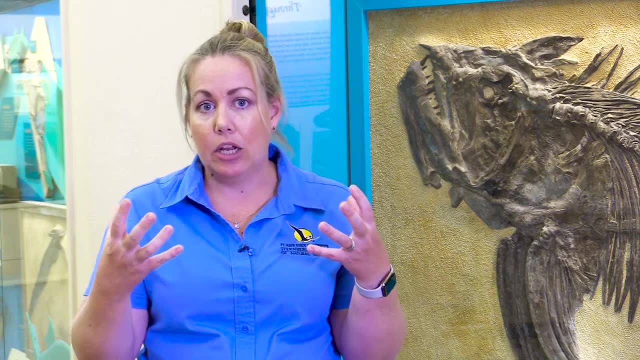 xipactinus for this. And if we look at the skull of the xipactinus, we see these big, powerful jaws with these really long and sharp teeth telling us that we quitting it's eating. you know big prey items, probably bigger fish we can also use. 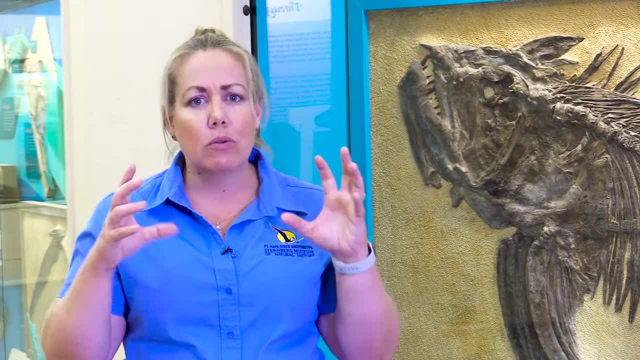 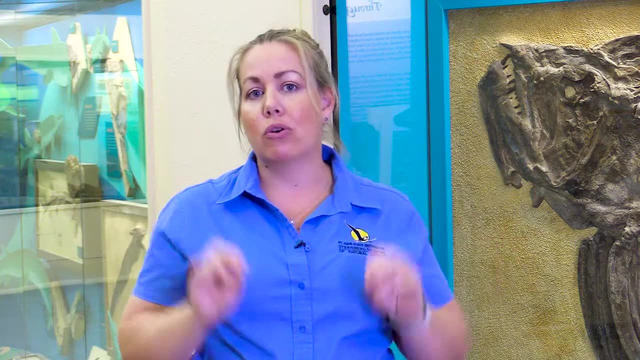 things like our gut contents to help. but then we can also look at how that jaw is put together and you can see it has this really strong lower jaw that actually has this little upturned snout on it, and so we actually think that this was a. 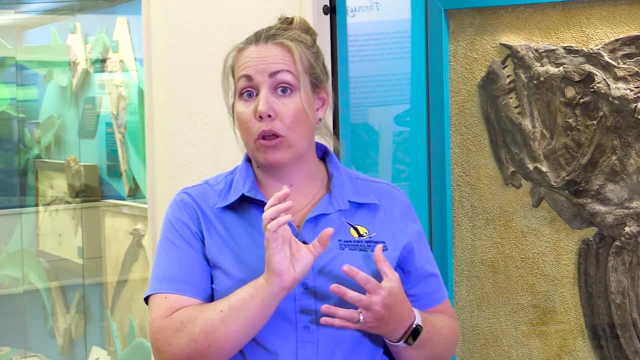 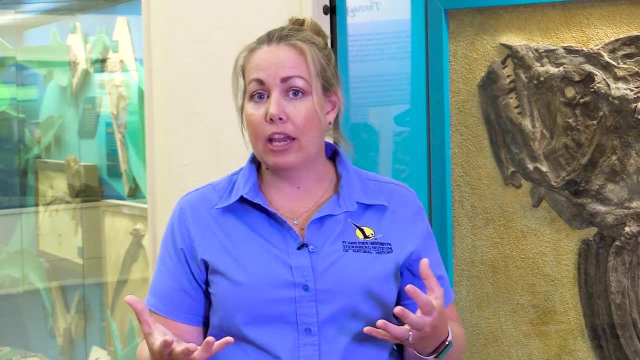 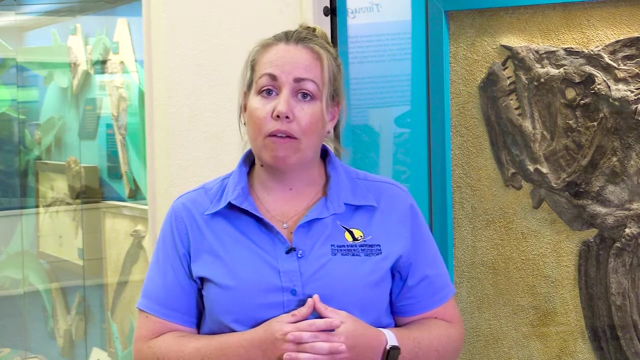 type of fish that would have been an ambush predator from below, and we know that again by putting together the shape and the size of skull and we can compare that to animals living today that look and probably functioned the same. and so looking at other fish fossils that we have within the fossil record of Kansas. 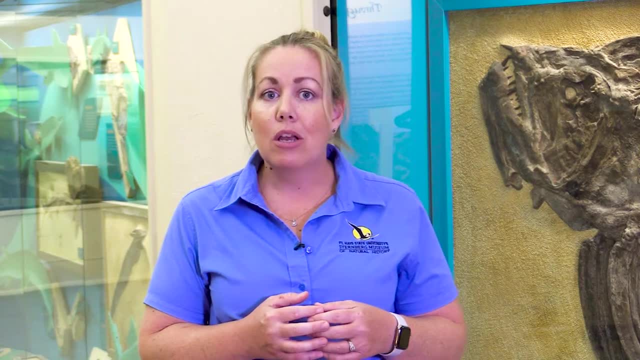 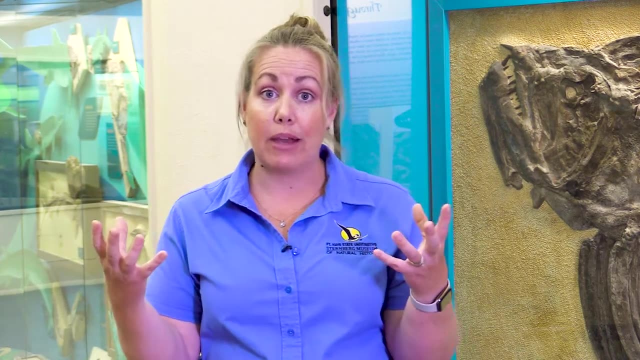 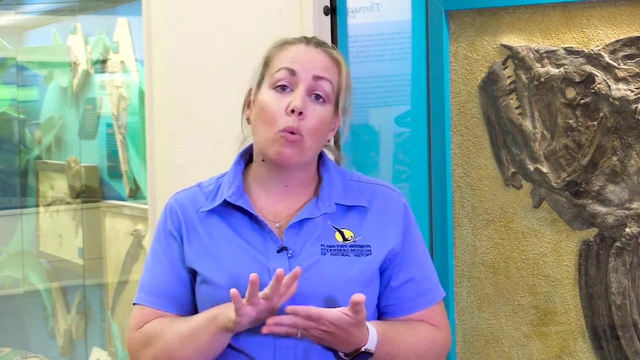 we can start putting together similar relationships so we can look at the shape and size of the head, how large the mouth would have opened, so maximum prey size, what the teeth looked like, whether they were used for grabbing, whether they were used for ripping or whether they were used for. 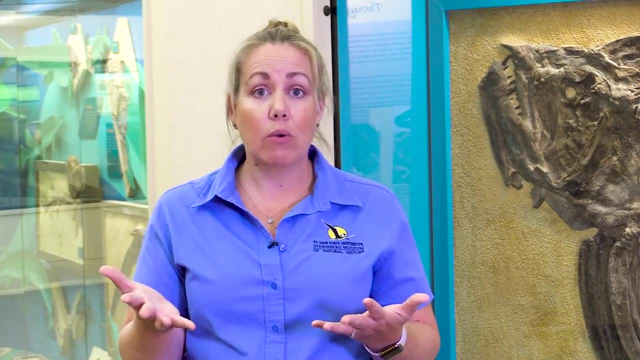 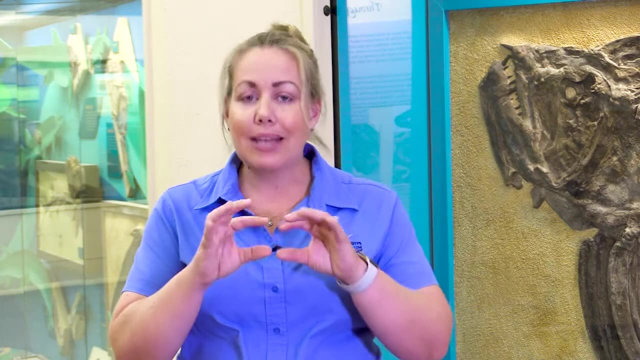 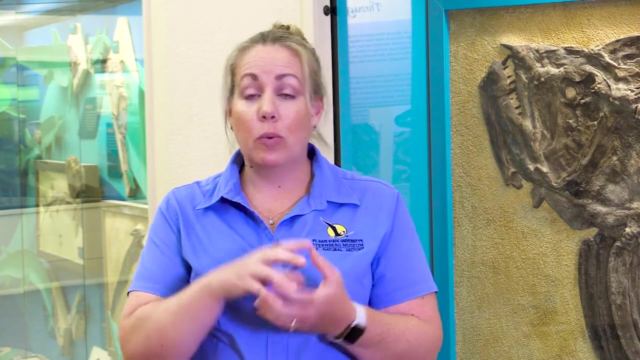 crushing. so we have a really cool type of shark called tychotis that would have lived in the same environments as our, as our xiphactinus and our gillicus, but it has these flattened, almost mushroom-shaped teeth that would have been used for crushing shells, and so we know that they weren't going to be used. 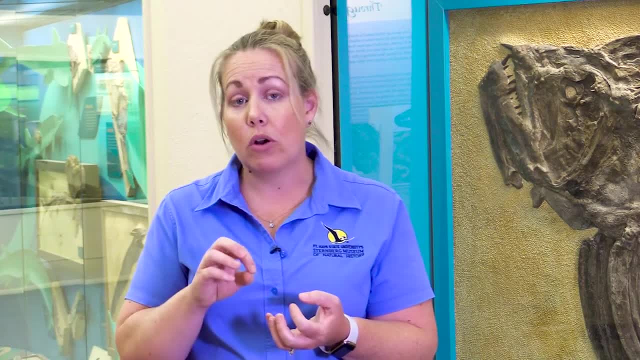 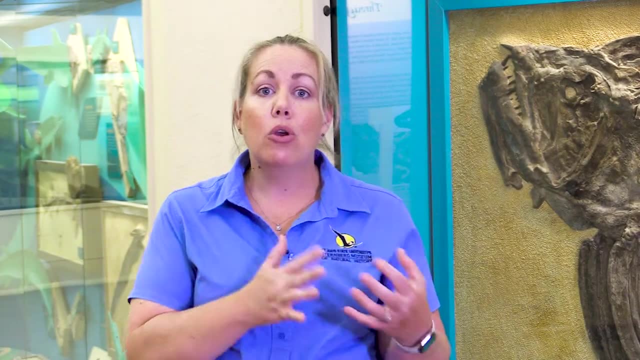 for really ripping, like we associate with other sharks, or or shearing, but again for crushing. so this gives us another ecological relationship. who was a fish? that was very skittish and very well done, but it would not be known that one is a eating whom, and this is really cool. so we can start to put together an ecosystem of the different. 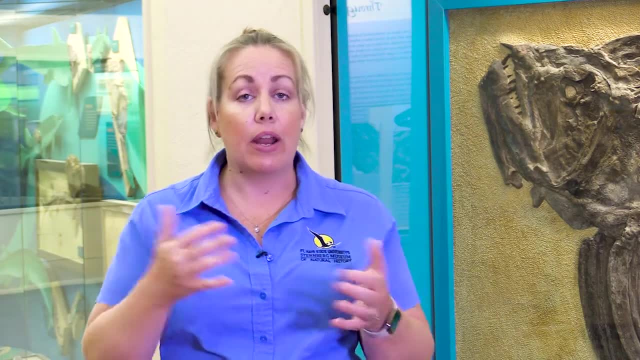 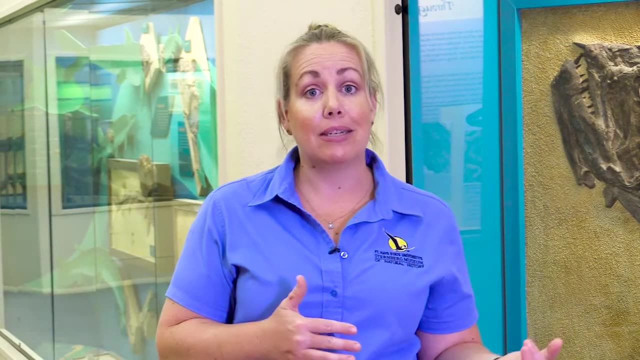 organisms, how they would have interacted with each other and how they would have fit into their physical environment together. and we can do things like: take that to the present and compare past ecosystems to the present. what's different, what's similar, how the climate was different, how it was. 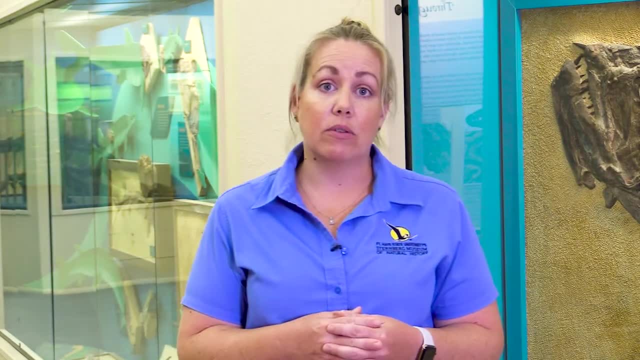 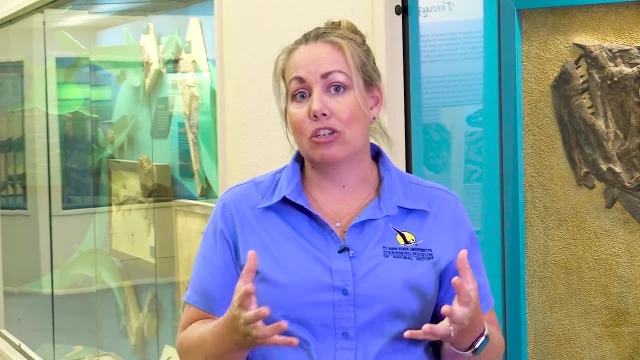 similar and how that could have influenced the different ecosystems. and then we can also take that into the future, and that's one of the really important parts of paleontology and science in general is kind of this ability to look at the past and predict the future. so all cool things. 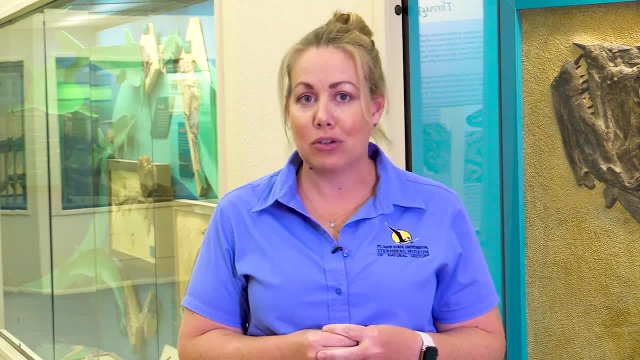 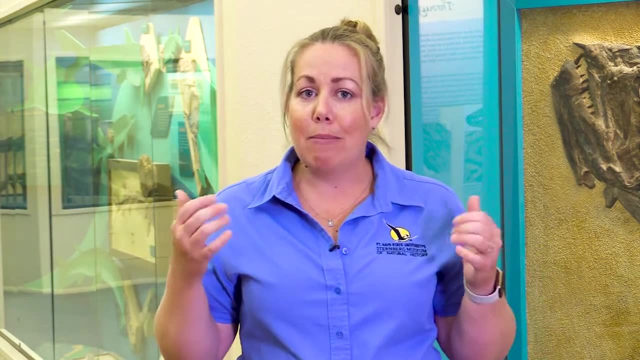 that we get to do as paleontologists, that we get to put together these fossil ecosystems, these ancient ecosystem, to ask and answer a lot of cool questions. so hopefully you liked this video. if you did give us a thumbs up, like us on social media, please leave us a comment and thank you for joining. 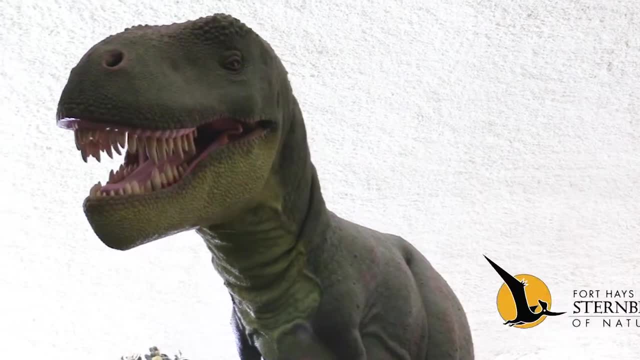 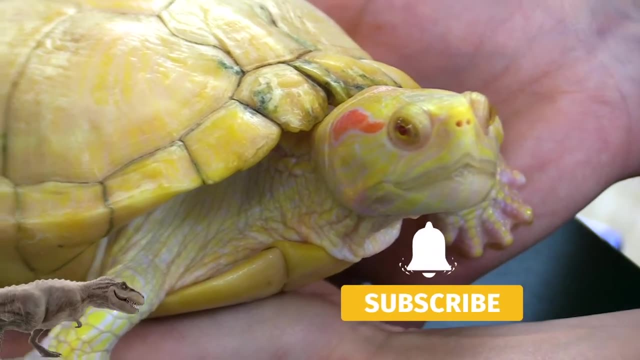 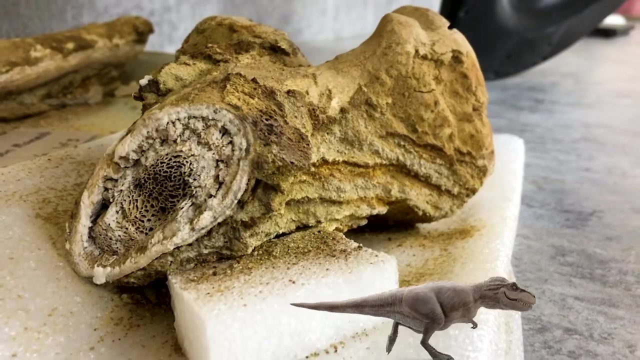 us this week for another new way to museum. thanks for joining us in a new way to museum with the sternberg museum of natural history. if you enjoyed this video, like it and subscribe to our Channel. hit the bell for notifications when we release a new video. support us on patreon for early access and exclusive content. you can also follow us on all. 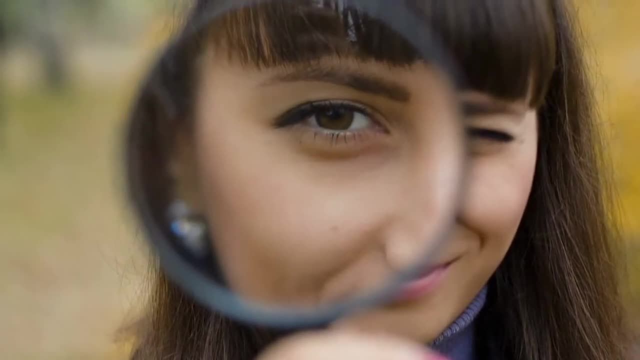 our social media links are found in the description. thanks for watching and follow your curiosity to new discoveries.